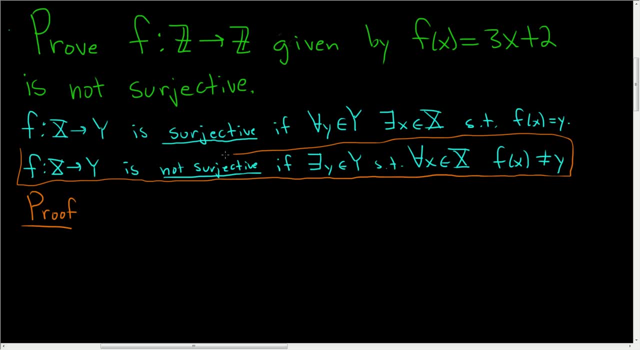 all we have to do is produce a value of little y in the codomain. So this is the codomain and this is the domain. They're the same in this case. It's a pretty easy problem. So we have to show the existence of a y. So let's go to the side and try to figure that. 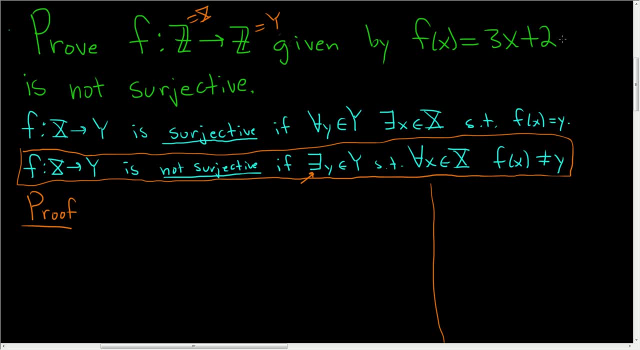 out. We need a y value such that f of x is not equal to y. So this is the set of integers. This is the set of integers. So we have to think of an integer such that 3x plus 2 is not equal to. 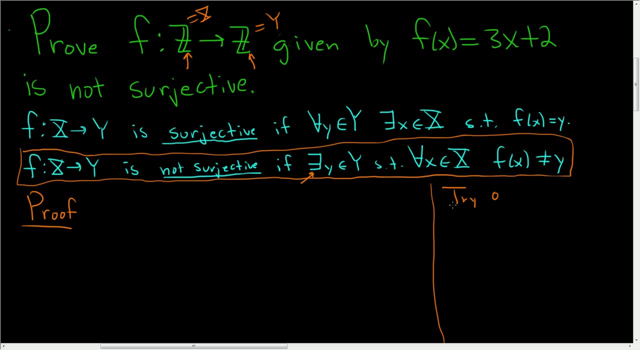 0.. So we're going to try that again. That would be x to the power of 4.. But then, as we go through this whole process, we can propose f of x as a integer. So let's look at the integer, Let's try. 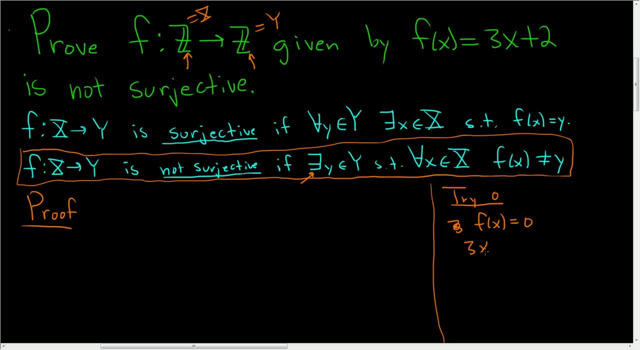 0.. Why 0?? Well, 0 is the easiest one to try. So is it possible for f of x to be equal to 0?? Let's see: Well, 3x plus 2, could that be equal to 0?? Well, if it was, then we would subtract 2 and we would. 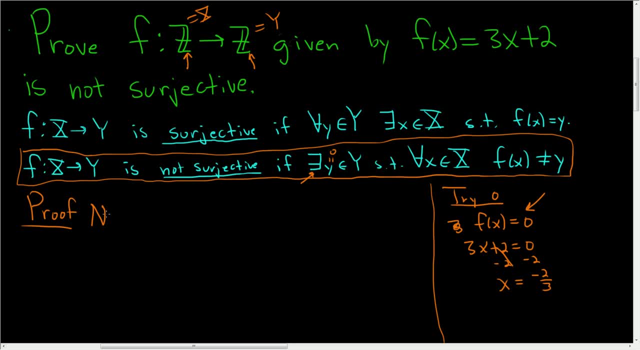 get x equals negative two-thirds, So we should be able to use 0 as our y in our proof. So note is: equal to zero is in capital Y, which is the set of integers, and f of X is not equal to zero for all X and capital X, which is the set of integers. so we're 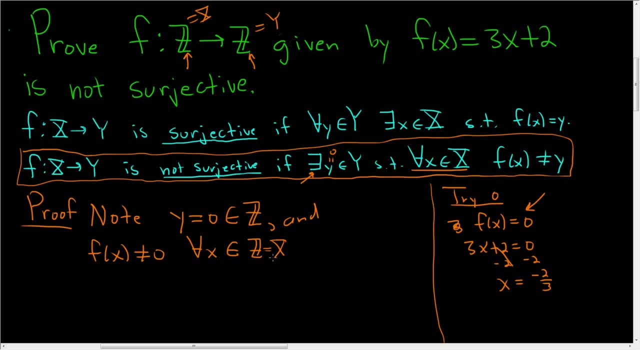 using this here. this is our, our capital X, this is our capital Y. so we showed the existence of a Y in capital Y and now we're saying that f of X is not equal to Y. this is our Y for all X in the domain. now, if that doesn't seem like a proof, 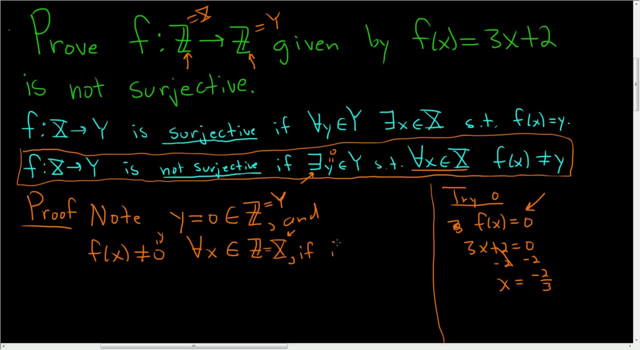 well, we can add more to it. we can say something like: if it was, and then prove it by contradiction, then we would have f of X equal to 0, which implies 3x plus 2, because f of X is 3x plus 2 equals 0, so X is equal to.